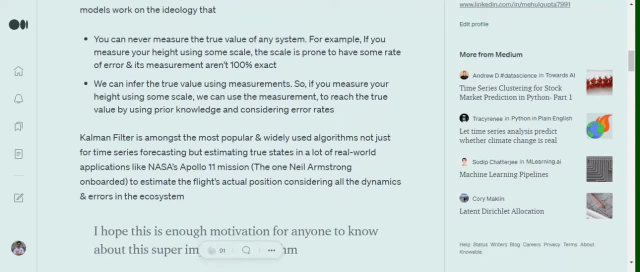 series forecasting, but also for correction of values, also assuming true states, of lot of real world entities. So if you might be a bit shocked to know that this algorithm was used for NASA, by NASA, behold soil analysis at the Apollo 11 mission, where Neil Armstrong landed on the moon, 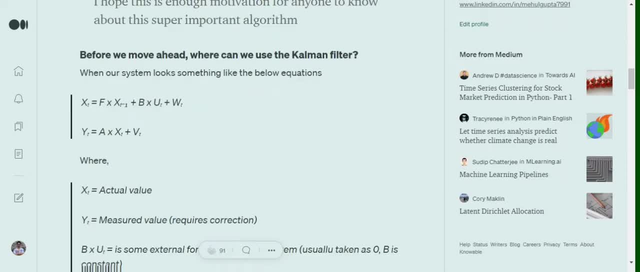 so this algorithm is very, very important. First of all, let's understand where we can apply the Kalman filter. The Kalman filter can be applied when our system satisfies the below two, the two equations that I mentioned. that is, Xt is equal to Fxt-1 needs to ext- 1. 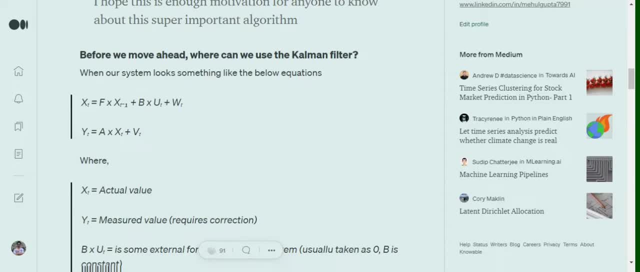 further, can apply the Kalman filter 0 plus b into UT plus WT and YT, 0, Ft-1 and KsSo and yt equals to a into xt plus vt. now let's understand what are these terms. so xt is the actual value actually, without any error, without any uh measure, and it's the correct, the most. 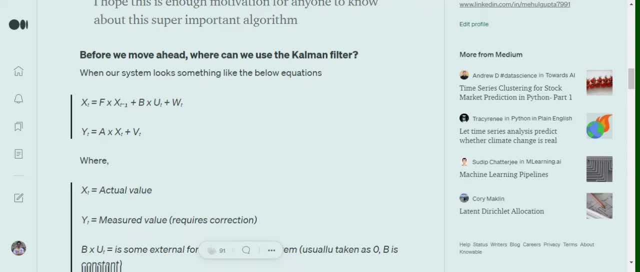 correct value that you can get now: f, b, a the equation, in the equation that i've been used, they're all constants. there are some weights present. xt minus one is, like again, a value back from a timestamp. ut is some external force that is working on. uh, so like in case of like, 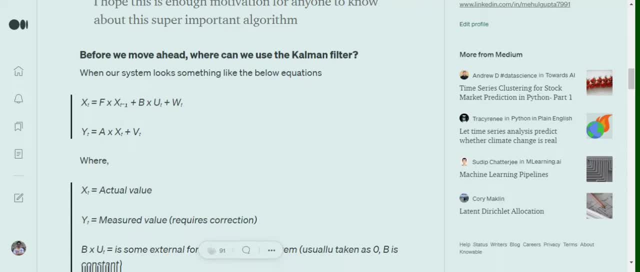 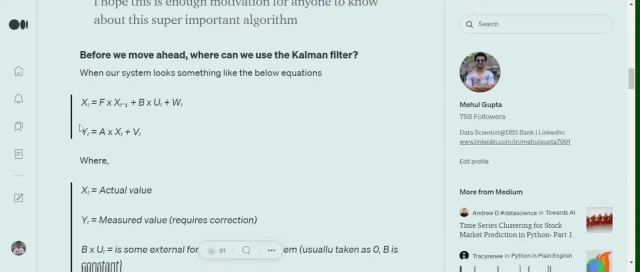 for example, when you're measuring a height, it can be the temperature, the gravity. it's an external force that is working. wt is some random error, stochastic, random that they call it now. yt is the measured value right and vt is the measurement error. so like, for example, when we're measuring our 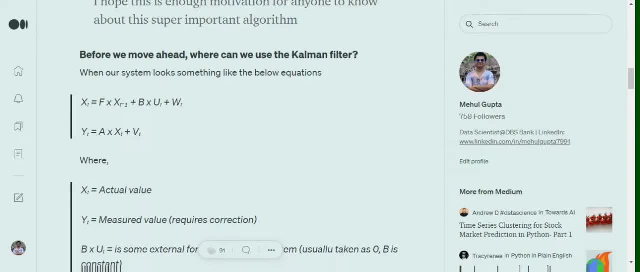 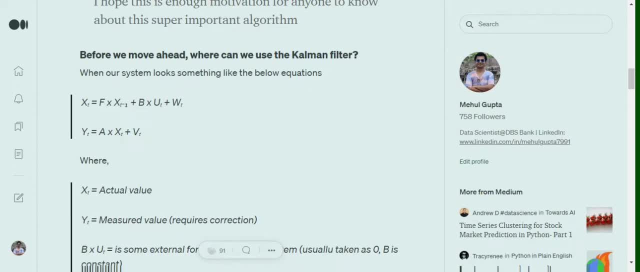 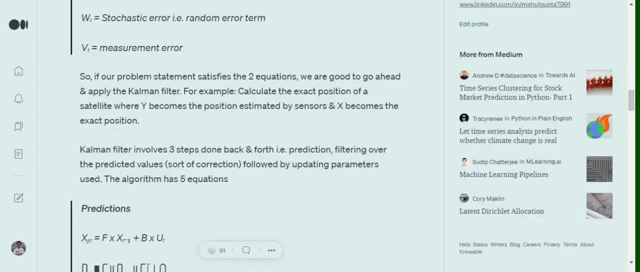 need to understand this equation, like they don't have any correlation between and. these equations are not related to each other, they're just the and your environment must satisfy these two equations to move ahead to use the kalvin filter. now let's understand how the kalvin filter works. 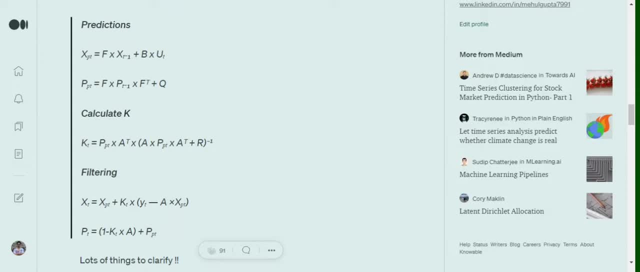 what are the equations involved? so the kalvin filter can be divided into three parts: one is the predictions, other is the calculating the kalvin filter constant and third is the filtering part. filtering part is majorly the correction part that we are calling about. so in prediction uh we have the values: xpt equals to uh, f cross xt minus one, plus b cross ut and ppt equals. 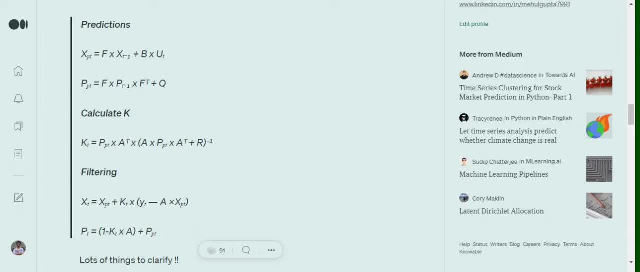 to. we are calculating two variables: xpt and ppt. uh, now, xpt and ppt are the predicted values- can be called as a measured measured value as well. so in uh, like in different scenarios, it can be different values. only in terms of time series we can call it as a measured value. so in terms of 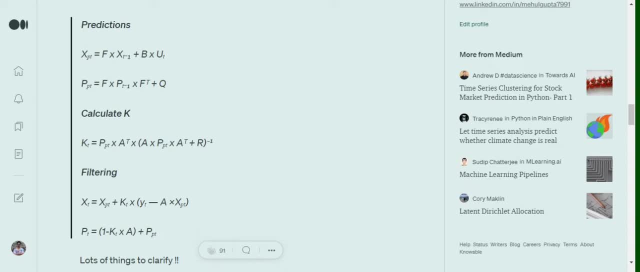 time series, we can call it as a predicted value and later on we will be filtering out to get the actual values right. in case of when you're measuring, a weight can be called as a measured value and when we're applying the filters, it will be called as an actual value. so xpt, is that, yt that? 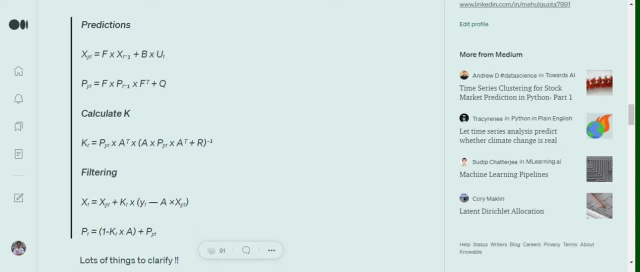 we are talking about right, the pt term, that pt subscript that has been applied, is the more of the yt terms that are getting predicted by the system but are not the actual values. as we said that values can't be measured ever, the real values can't be measured ever. now, in this equation, pt is the. 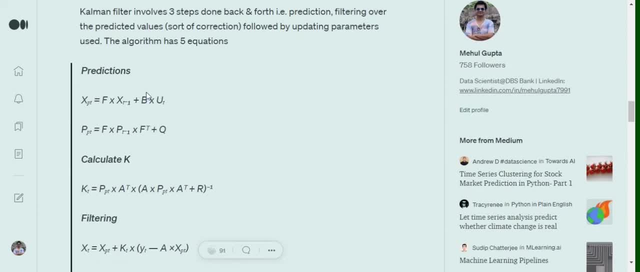 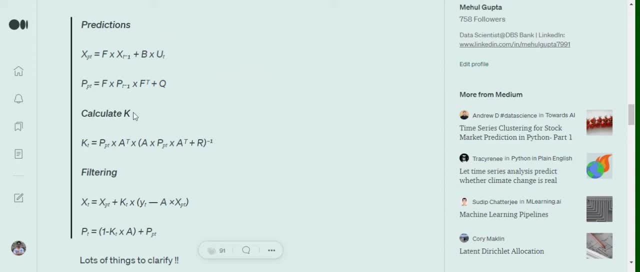 covariance metrics of the error terms. uh, this is something that i haven't discussed yet, and i really couldn't find out much on it on the internet as well. uh, now, next we calculate the kalman filter using all these variables. i will discussing what are these variables. these are tough equations, so explaining. 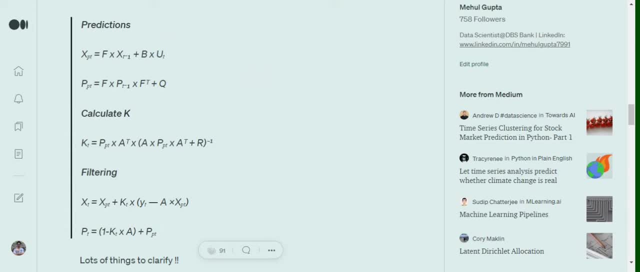 this equation won't make any sense. we will explain the terms that have been used and then the filtering part. so the filtering part: you can see that how the predicted values are used to get to the final value and the predicted value. you can see that we are using the predicted value. we are 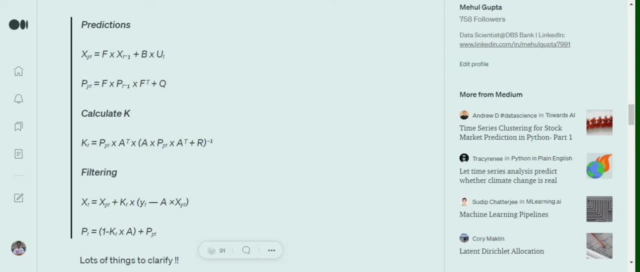 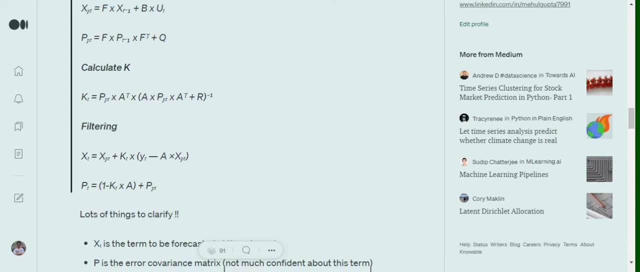 also using kalman filter or the kalman filter constant. that has been calculated and also the measured value as well. and pt uh is again getting updated. that is the error covariance matrix. so if you look, look into it, x is the term to be forecasted at timestamp t. 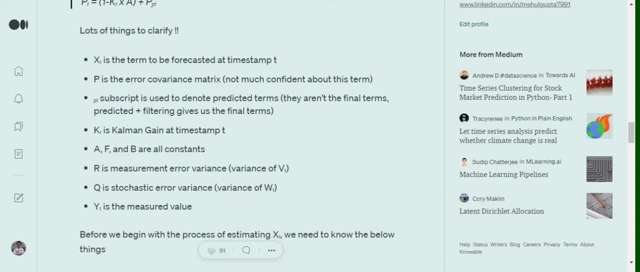 forecasted or the actual values that we wish to get. it's the final one that we wish to get. p is the error covariance matrix and nothing i really couldn't find much about on the internet. pt is a subscript used to denote predicted terms. they aren't the final terms, as i said you earlier.